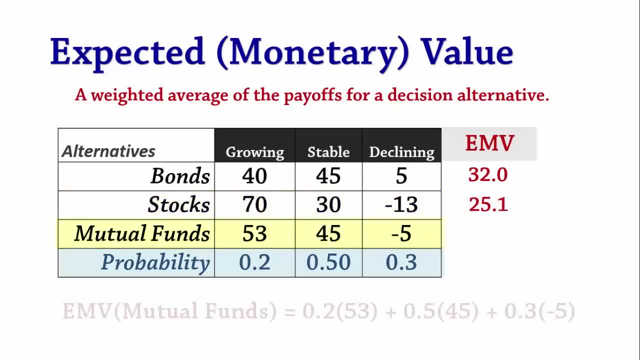 which equals 25.1.. For mutual funds, the expected value is 0.2 times 53 plus 0.5 times 45 plus 0.3 times negative 5, which equals 31.6.. The best expected value is 32.. Therefore, 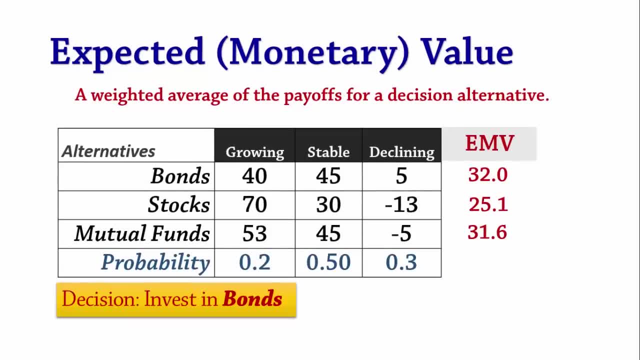 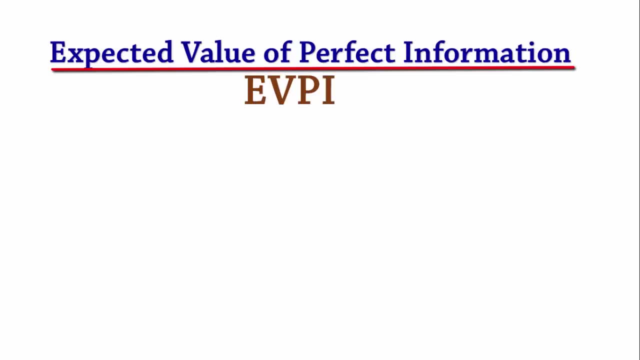 the decision is to invest in bonds. Expected Value of Perfect Information. The Expected Value of Perfect Information is the maximum amount you will be willing to pay for additional information about a decision. problem, That is, if we have perfect information about the state of nature before the decision is. 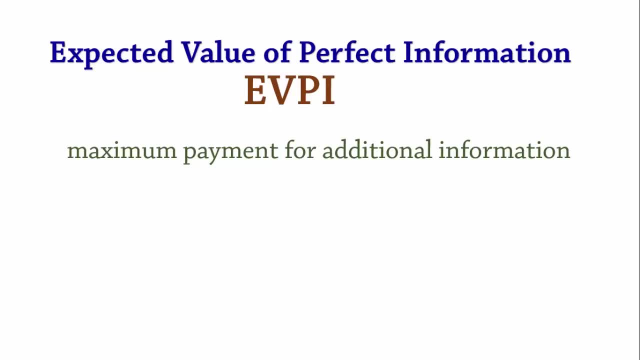 made. how much is this information worth? The formula for the Expected Value of Perfect Information is: eVPI equals eV with PI minus eV without PI. eV with PI is the expected payoff if perfect information about the state of nature is known. eV without PI is the expected value without. 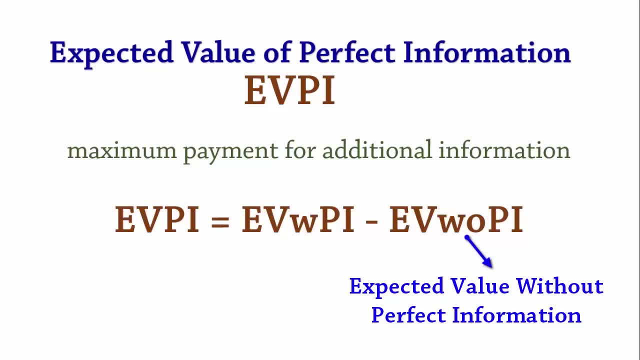 perfect information. So eV with PI equals eV with PI equals pI and pI is the most expected value. That is, eV with PI equals pI is the maximum eMV. The maximum eMV was determined to be 32 earlier. 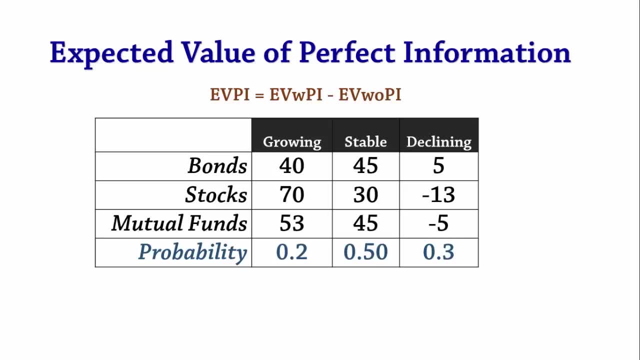 To calculate eV with PI ie Expected Value with Perfect Information, we choose the best payoff for each state of nature and multiply them by the probability of their state of 70 times 0.2 plus 45 times 0.5 plus 5 times 0.3, which equals 38.. 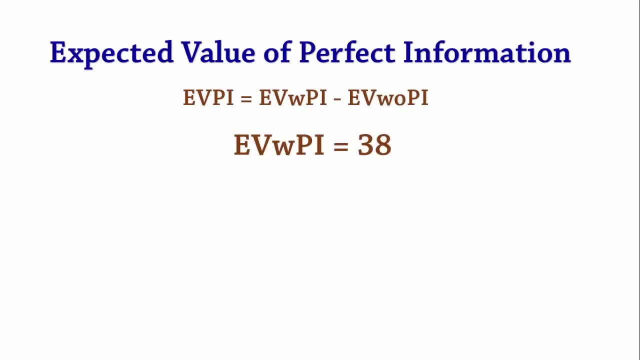 The expected value with perfect information is 38.. As calculated earlier, the expected value without perfect information or maximum EMV, is 32,. therefore EVPI is 38 minus 32, which is 6.. So if we have perfect information about the states of nature before the decision is made, 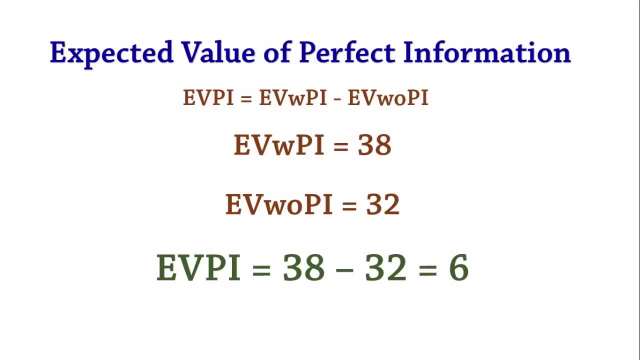 the expected value of that perfect information will be 6.. And that's how you calculate EVPI. Thanks for watching.